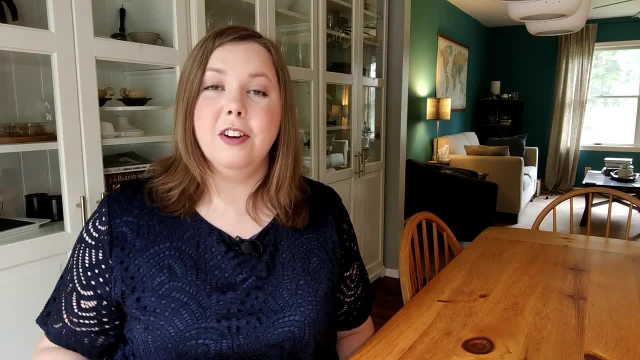 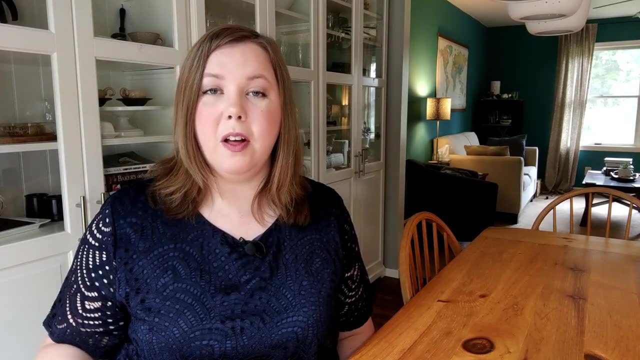 things that go into why a product is or isn't selling, from whether the features meet the needs of the consumer, to marketing, to competitors' products that are available, and all of these really need to be addressed to figure out how to sell more product. 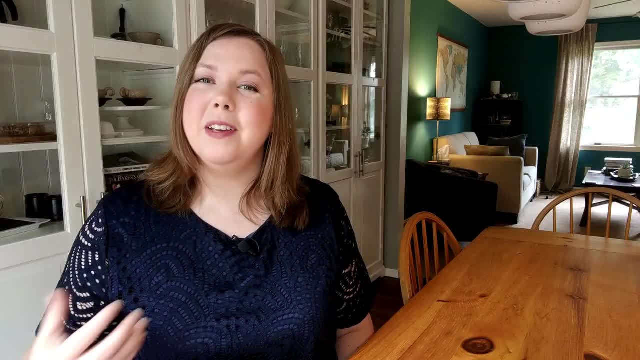 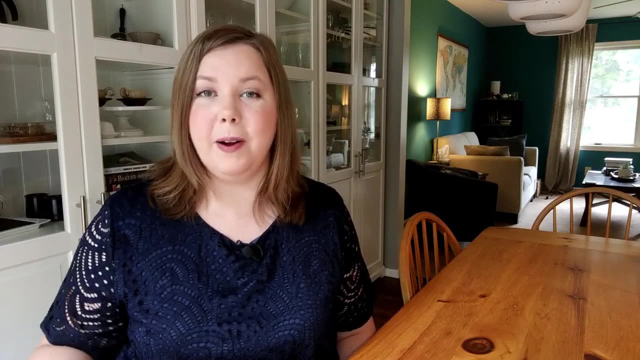 Here, the real problem is: how do I sell more product? We still need to analyze pieces of that. so one of the pieces of deciding how to sell more product is certainly going to be: how is the product priced? One key to being a good analytical thinker is knowing when you 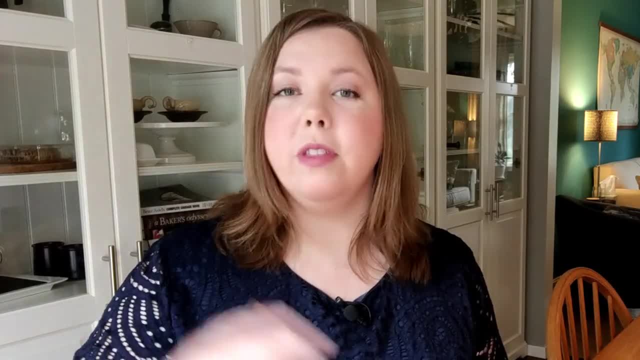 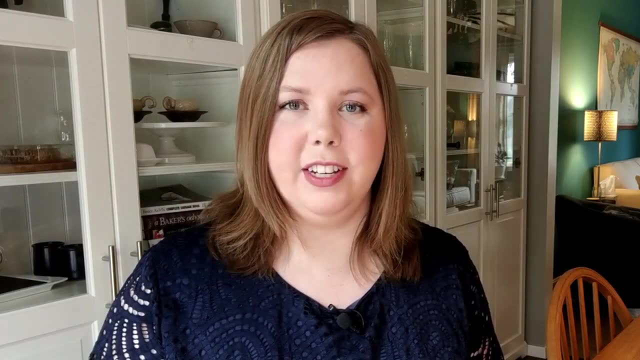 are only solving one part of the problem. So if you know that the bigger problem is how do we sell more product, then you can talk about price in the context of that question. Once we've identified the problem, the second step is to decide. 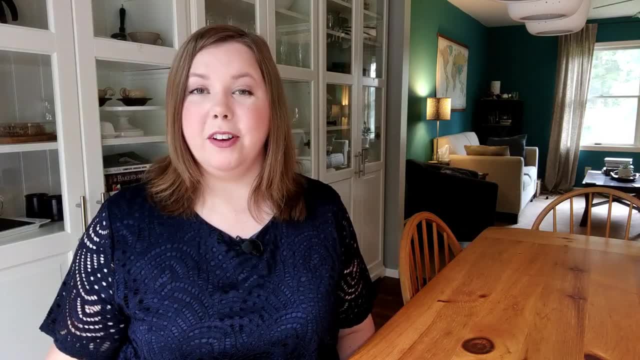 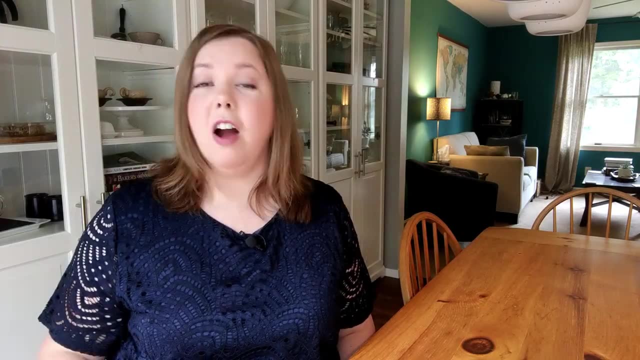 how you're going to go about solving it. Here we're setting up the problem-solving approach. What tools, techniques or methods are you going to use? What data do you need to be able to solve the problem? Are there people that you need to be involved in solving this problem, or do you? 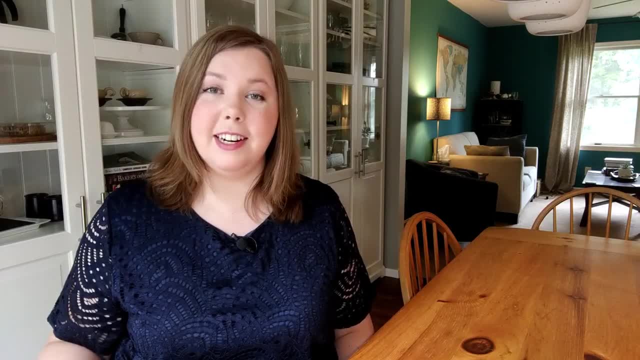 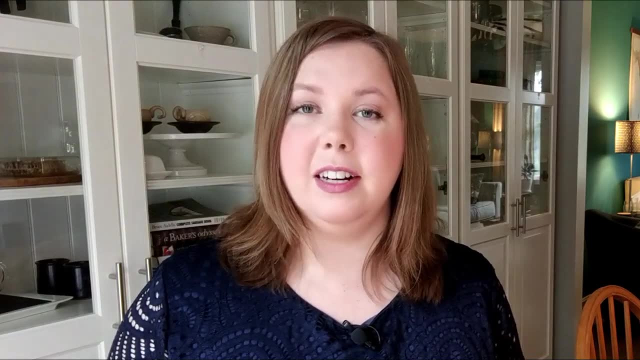 have all of the resources available to you that you can figure out entirely on your own. Establishing a good strategy to approach the problem makes the entire solving process easier. It lets you go through a lot of the logical thinking of how to solve it. 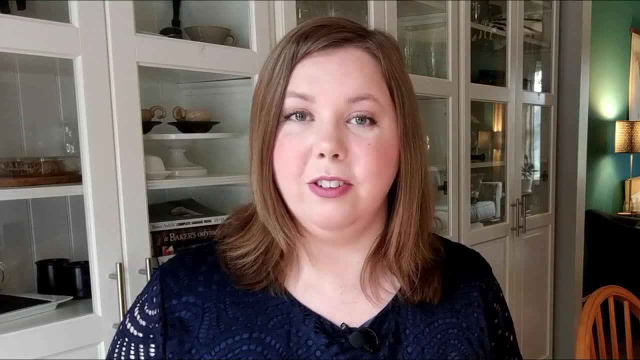 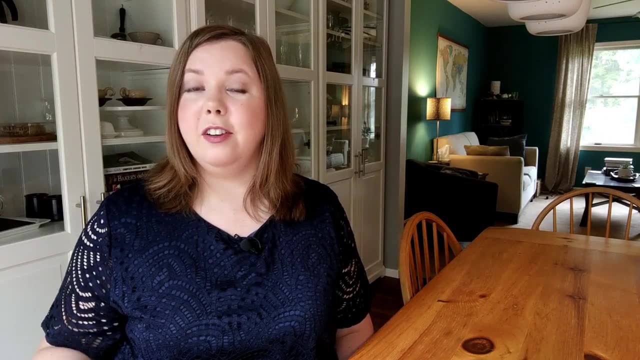 and then supplement with the information you need to actually get that solution. At this stage, you can also consider whether to break the problem into multiple parts. For instance, if you identified your problem as how do we sell more product, you may identify a. 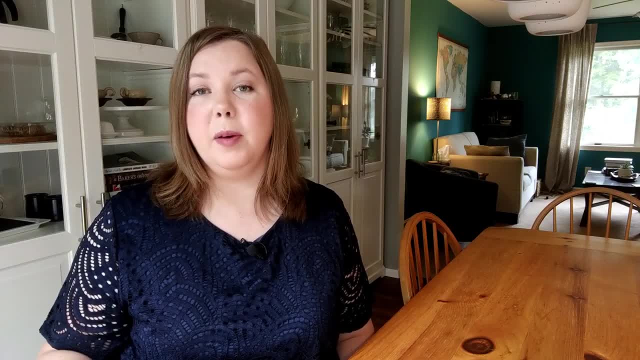 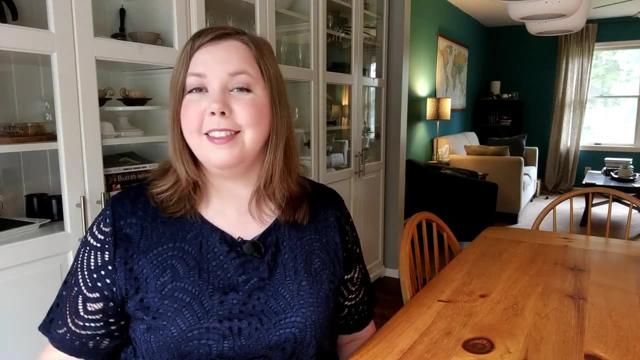 half a dozen different things that need to be analyzed or solved to be able to complete that answer, One of which is pricing, one is marketing, one would be competitor products, and the list goes on. These first two steps are going to help you figure out how you're going to solve the problem. 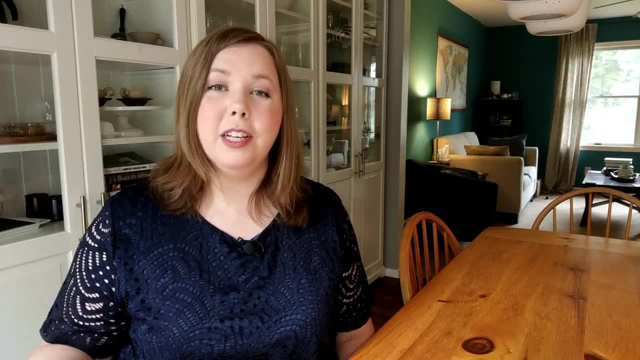 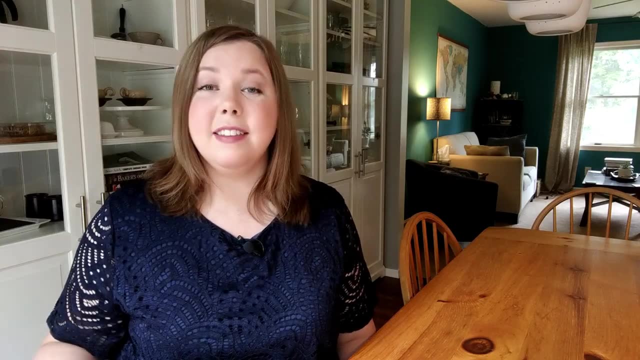 The first two steps might make it sound like analytical thinking is really only for mathematical problems. Analytical thinking can be used for even non-math problems, though. You can examine the data even if it's not numerical data. We do this all the time with.